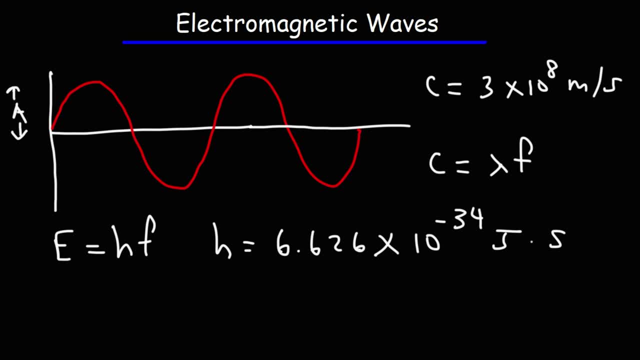 Now there's a lot of different types of waves in nature. Think of an ocean wave. You know it has a crest, It has a trough. Think of a wave on a string. But an electromagnetic wave is different. This type of wave is composed of electric and magnetic fields. 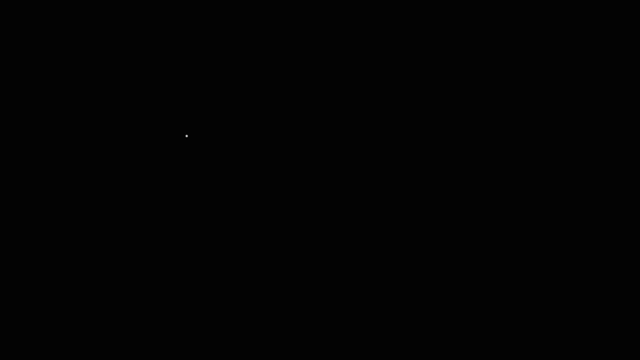 Thus we have the name electromagnetic waves And let's draw it. So we're going to draw a 3D coordinate system. My drawing's not perfect, but I'm going to make the best of it. So first let's draw the electric field component of an EM wave. 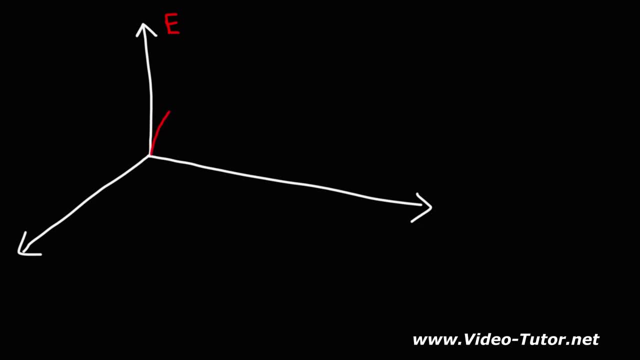 The electric field oscillates up and down. We'll call this axis time. Now, when the electric field is changing, it will create a change in magnetic field, And the change in magnetic field in turn will create a change in electric field. 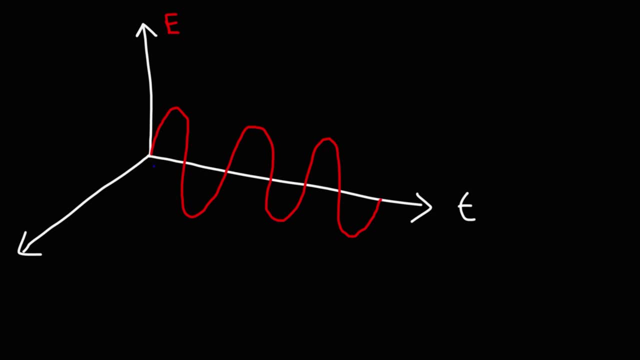 And so when you're dealing with an EM wave, you have an electric field on one axis And perpendicular to it you have a magnetic field. We'll call it B. So that is an electromagnetic wave. On one axis you have the electric field, which are oscillating. 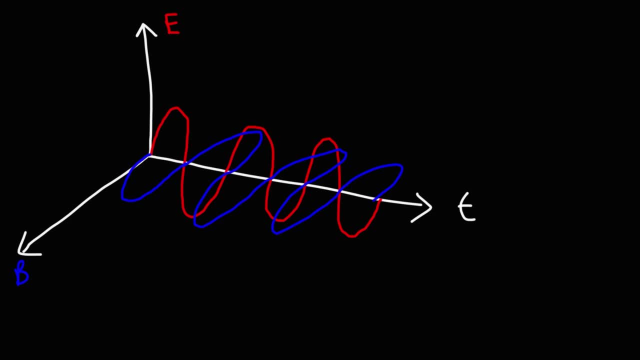 And on another axis, perpendicular to it, you have oscillating magnetic fields. The electric field is equal to the speed of light Times. the strength of the magnetic field. Electromagnetic waves can be created by any type of charged particle. A charged particle always has an electric field around it. 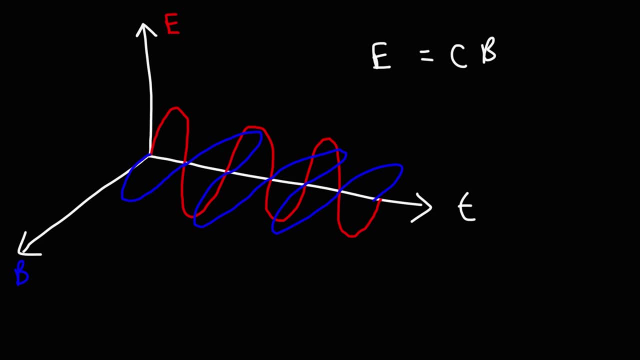 A moving charged particle can create a magnetic field, But an accelerating charged particle can create a propagating electromagnetic wave. Here's another example. So let's say we have a hydrogen atom And let's say that this is the first energy level. This one is the second. 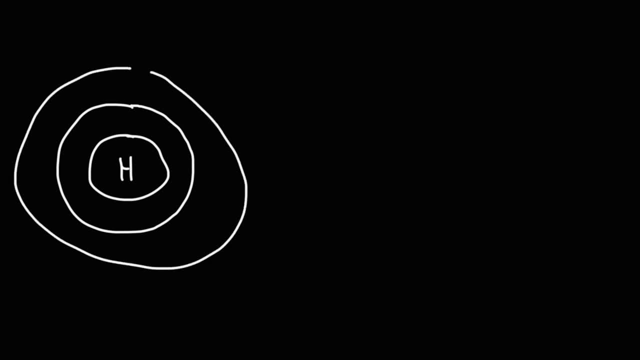 And let's say this is the third energy level. Let's say we have an electron, An excited electron, in a third energy level. When the electron drops from the third energy level to the second energy level, Or even lower than that, This makes a new energy level. 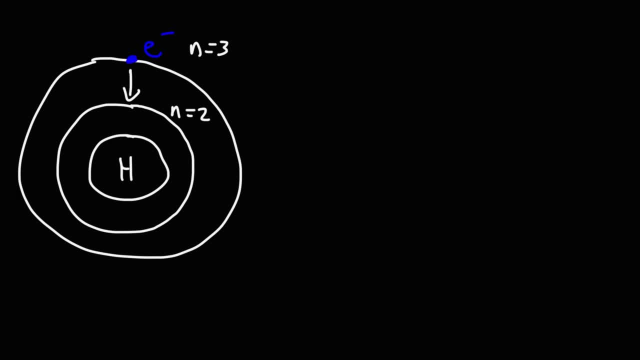 Now, any time it goes from a high energy level to a low energy level, it can emit an electromagnetic wave. Sometimes it can emit a photon of light. Now for the hydrogen atom, the energy of the photon that's emitted is equal to negative 2.18 times 10, to the negative 18 joules times 1 over n final squared, minus 1 over n initial squared, where n is the energy level of the electron. 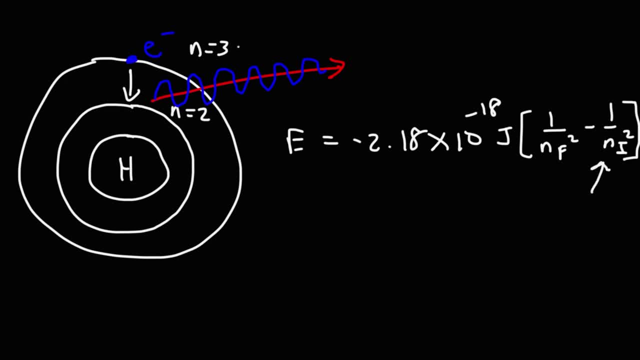 This is the initial energy level. In this case, that would be n equal 3.. This is the final energy level. That's where it's going to n equal 2.. When an electron absorbs a photon, it can jump from a low energy state to a high energy state. 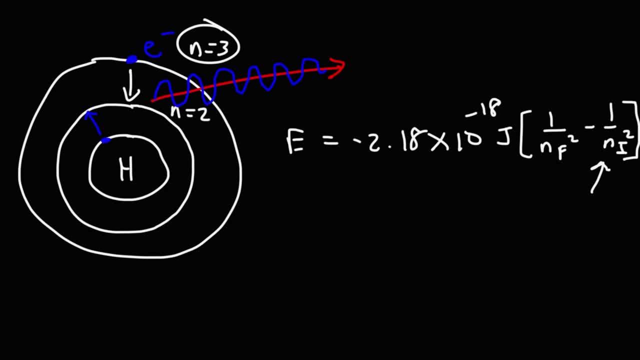 But when it falls from a high energy state to a low energy state, it can release a photon in the form of an electromagnetic wave. But not only that, though. when electrons are oscillating within a metal, they can also emit electromagnetic waves, even when they're heated. 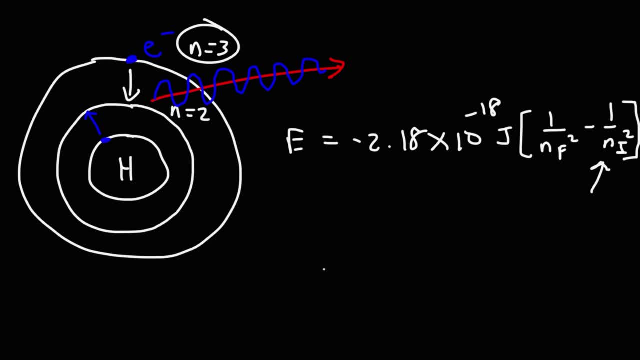 If you were to heat up metal to a very high temperature, it would emit electromagnetic waves. If you were to heat it up to a very high temperature, eventually the metal will appear red hot. If you were to heat it up to a very high temperature, eventually the metal will appear red hot. 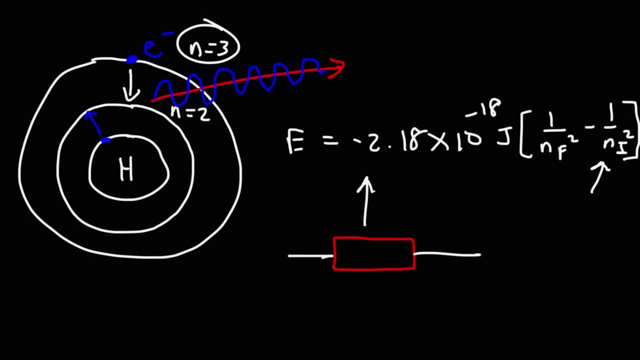 At this point it's emitted infrared radiation and even red light as well. As you raise the temperature, it'll produce light. through incandescence It'll appear yellow, and if you raise it even further, it'll appear bright white.